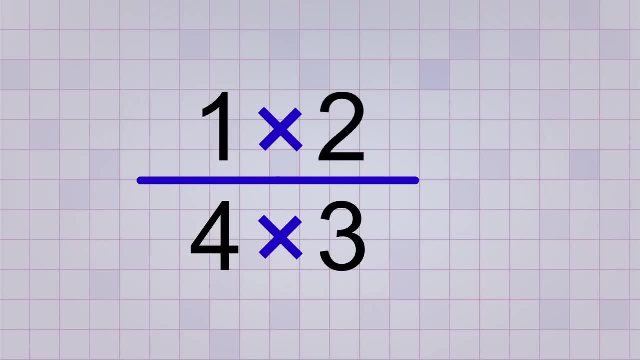 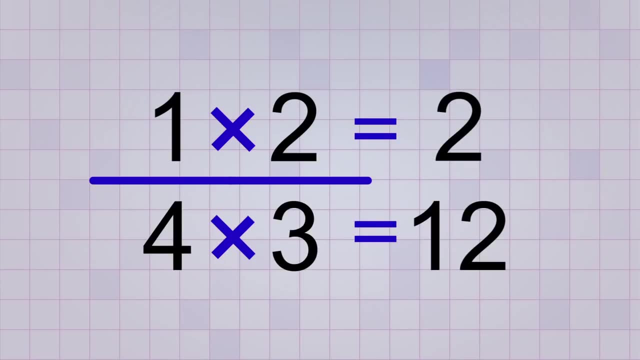 being divided and it looks just like a fraction. In fact, if we go ahead and do the multiplications, one times two equals two, and four times three equals twelve, then we do have a fraction and it's the answer to our problem. 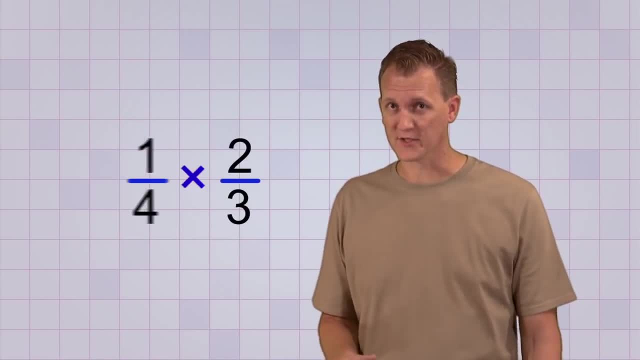 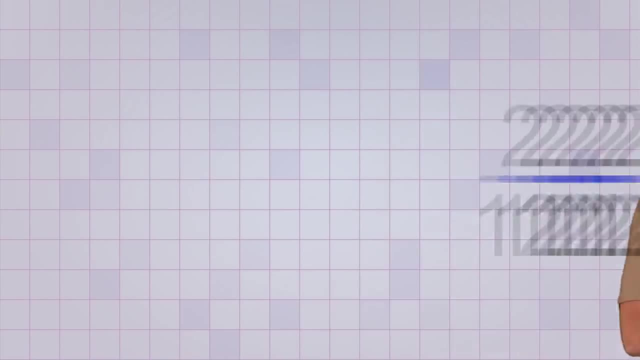 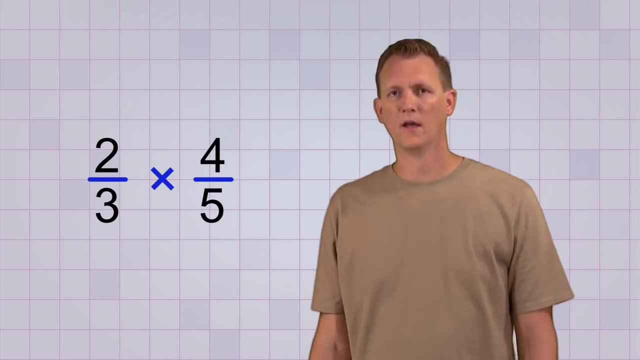 So what does all this mean? Well, it means that to multiply fractions, all you have to do is multiply the top numbers and then multiply the bottom numbers, and ta-da, There's your answer. As always, let's see an example or two. Let's try this problem Two-thirds times four-fifths. 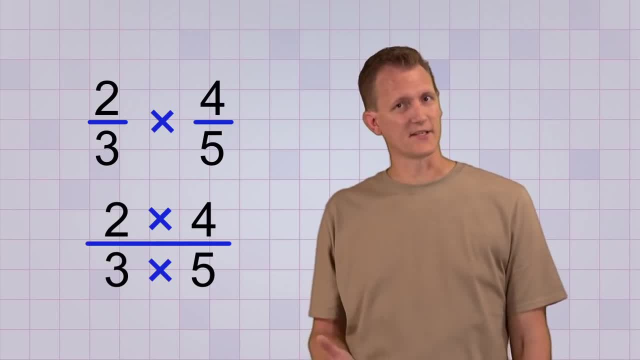 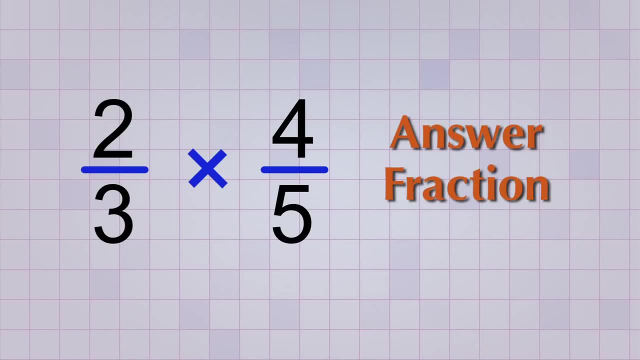 Now we could rewrite the problem like we just saw, but that's not necessary as long as we remember the procedure. First. we know our answer is going to be a fraction, so let's go ahead and write a new fraction line for it. 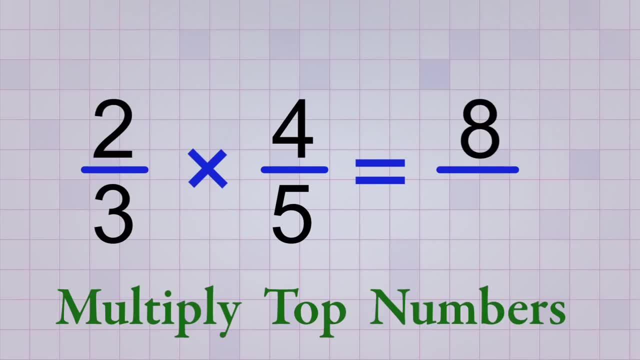 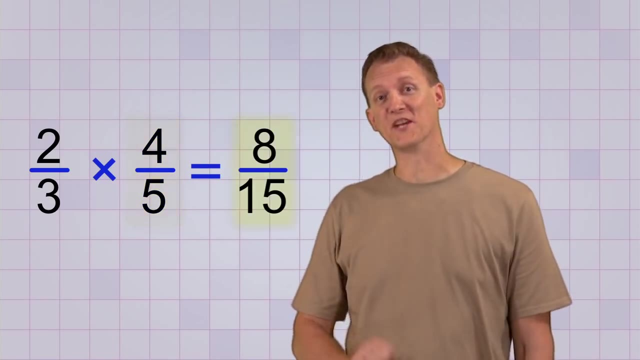 Next, we multiply the top numbers two times four equals eight, so eight's the top number of our answer. And last, we multiply the bottom numbers Three times five equals fifteen, so fifteen is the bottom number of our answer. There we have it. two over three times four over five equals eight over fifteen. See how. 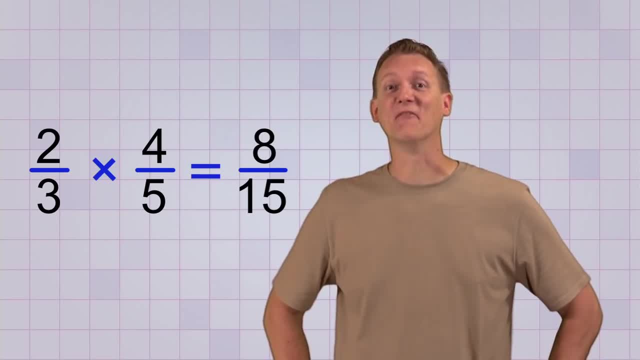 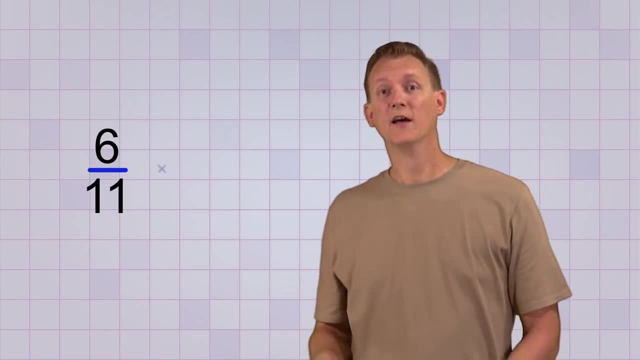 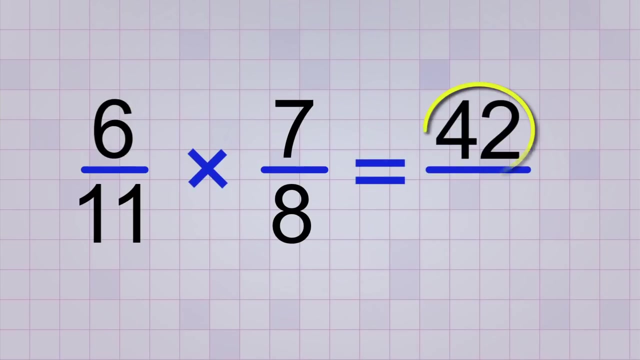 easy that was, And fun too, Even funner than video games. Okay, time for another example. Let's try: six over eleven times five equals five. Look, 11 times 7 over 8.. From our multiplication table we know that 6 times 7 equals 42. So 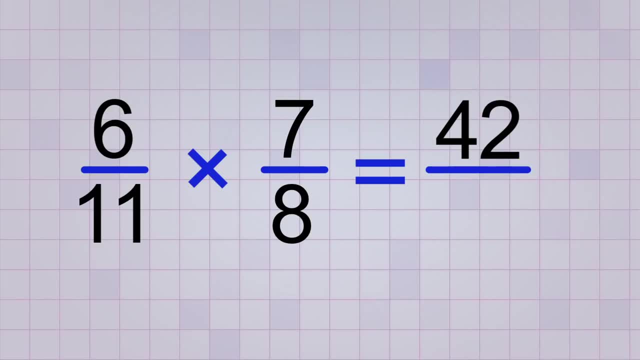 42 is the top number of our answer, And on the bottom we have 11 times 8, which is 88. So 6 over 11 times 7 over 8 equals 42 over 88.. Oh, now some of you might see that this. 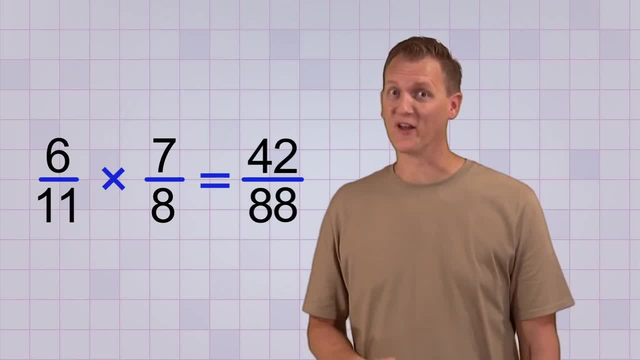 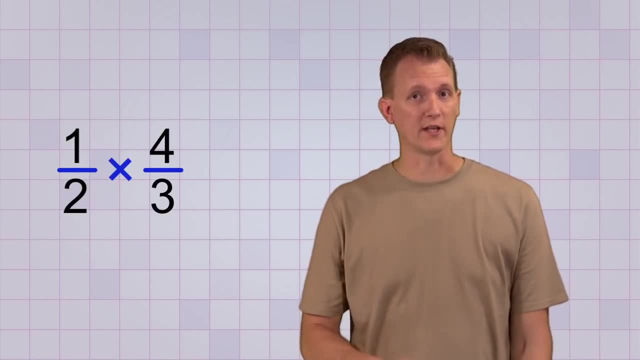 answer could be simplified, but we'll save simplifying fractions for another video. Alright, let's see one last example Here. it is 1 half times 4 over 3 times 3 over 5.. Wait a minute. This has 3 fractions multiplied together And the middle one looks like an. 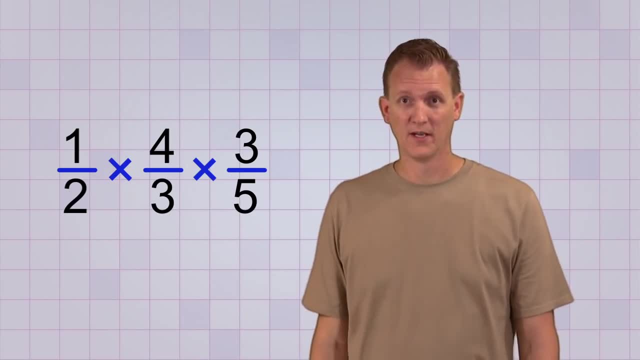 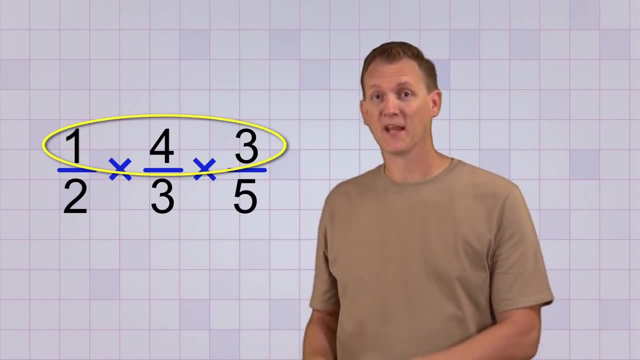 improper fraction because its top number is bigger than its bottom number. Does our procedure work for this problem too? Yep, All we have to do is multiply all the top numbers together and then multiply all the bottom numbers together, and we'll have our answer, And this will. 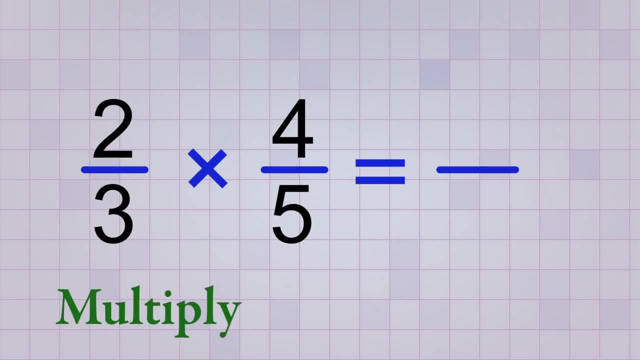 go ahead and write a new fraction line for it. Next, we multiply the top numbers Two times four equals eight, So eight's the top number of our answer. And last, we multiply the bottom numbers Three times five equals fifteen. 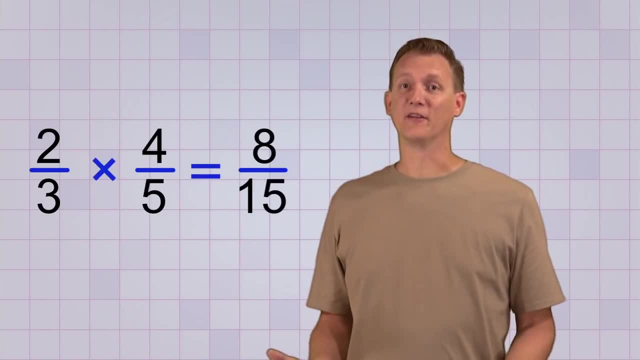 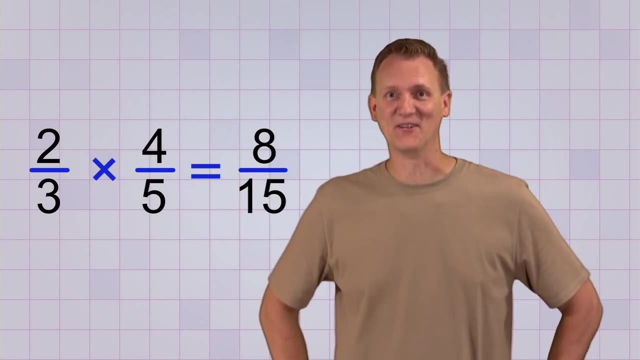 So fifteen is the bottom number of our answer. There we have it. Two over three times four over five equals eight over fifteen. See how easy that was, And fun too, Even funner than video games. Okay, time for another example. Let's try this one: Six over eleven. Six over eleven. 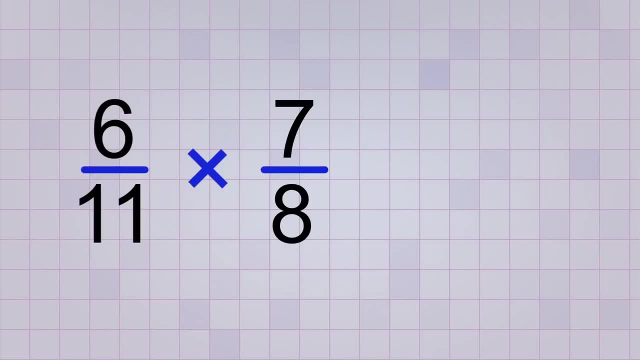 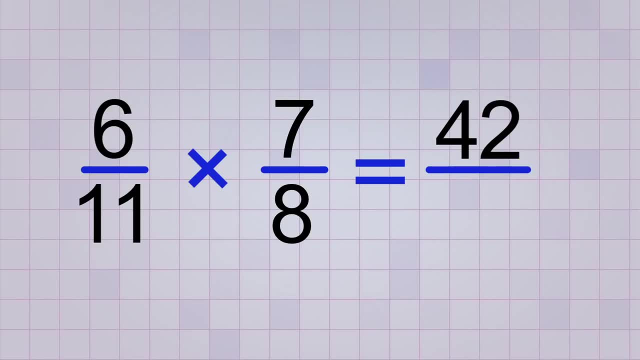 42 is the top number of our answer, And on the bottom we have 11 times 8, which is 88. So 6 over 11 times 7 over 8 equals 42 over 88.. Oh, now some of you might see that this. 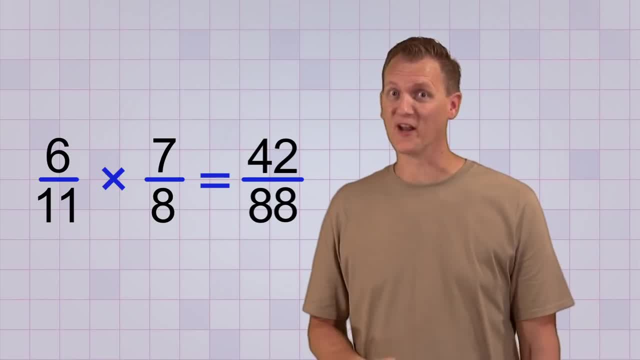 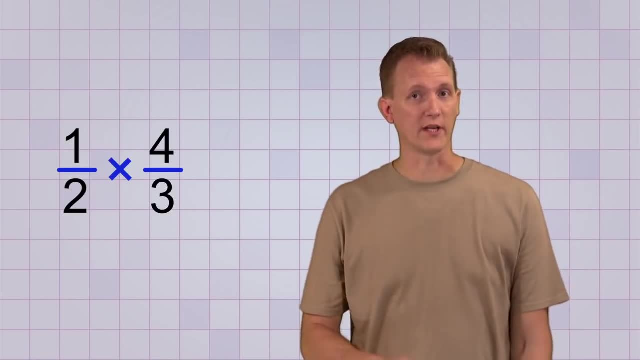 answer could be simplified, but we'll save simplifying fractions for another video. Alright, let's see one last example Here. it is 1 half times 4 over 3 times 3 over 5.. Wait a minute. This has 3 fractions multiplied together And the middle one looks like an. 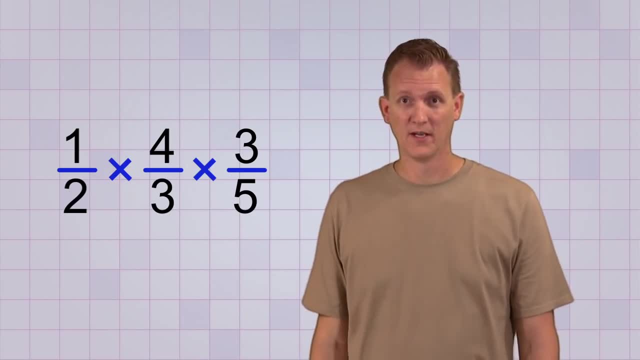 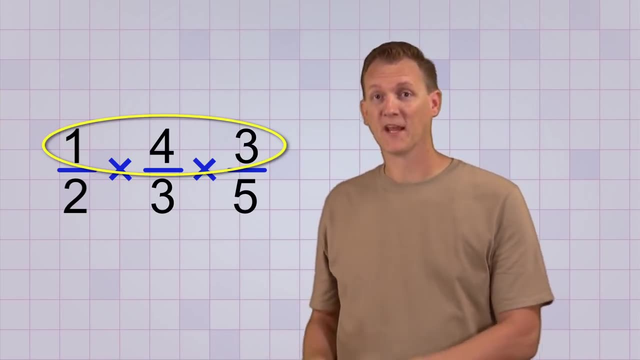 improper fraction because its top number is bigger than its bottom number. Does our procedure work for this problem too? Yep, All we have to do is multiply all the top numbers together and then multiply all the bottom numbers together, and we'll have. 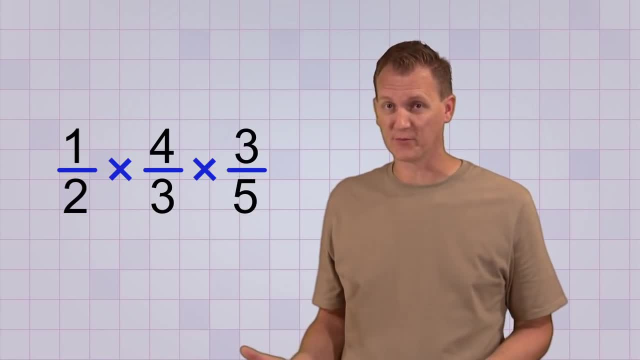 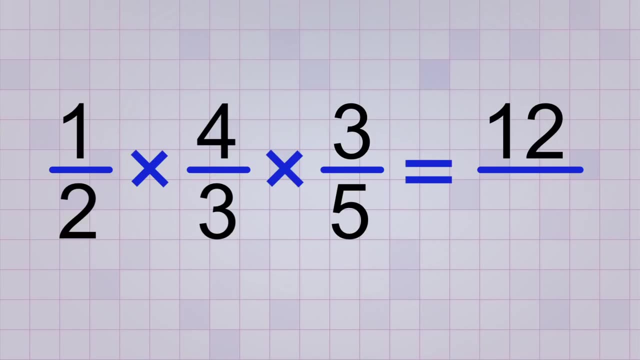 our answer And this will work no matter how many fractions we have to multiply. So on the top we have: 1 times 4 is 4, and 4 times 3 is 12.. And on the bottom, 2 times. 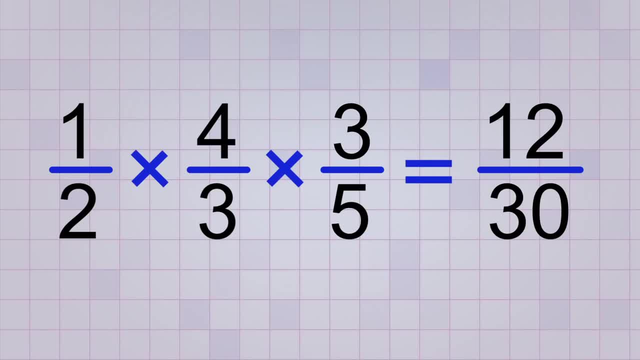 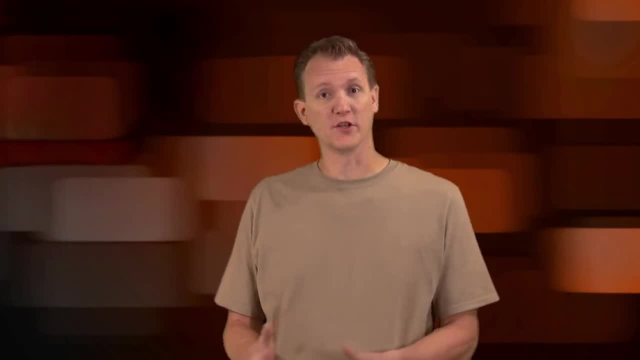 3 is 6, and 6 times 5 is 30.. That means our answer is 12 over 30.. So there you have it. Multiplying fractions is easy, because fractions are just another way of writing division problems. But remember, there's another way to think about fractions. 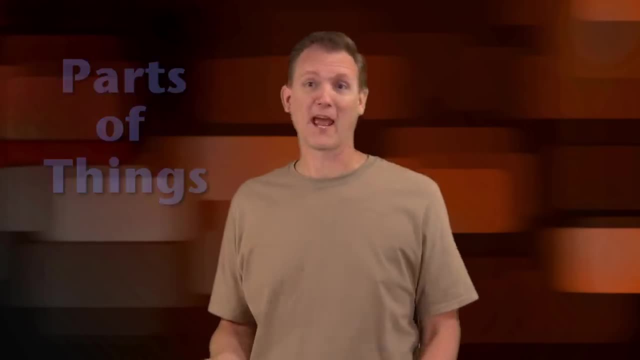 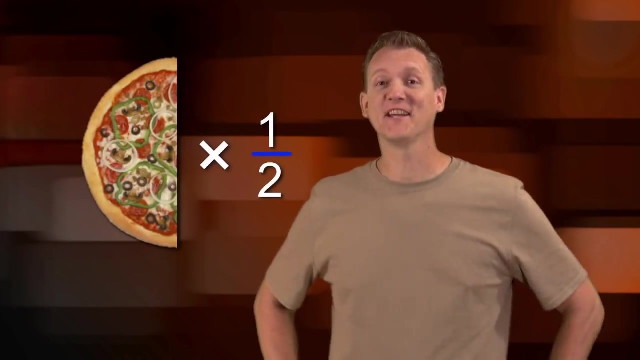 We can also use fractions to represent parts of things, like half a pizza, for instance, But does it make sense to multiply half a pizza by another half? Actually it does. If you're thinking of fractions as parts of something, then multiplying fractions is. 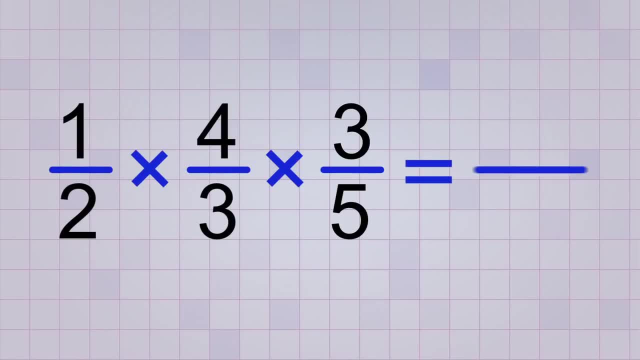 work, no matter how many fractions we have to multiply. So on the top we have: 1 times 4 is 4 and 4 times 3 is 12.. And on the bottom, 2 times 3 is 6 and 6 times 5 is 30. That means our answer is 12 over 30.. 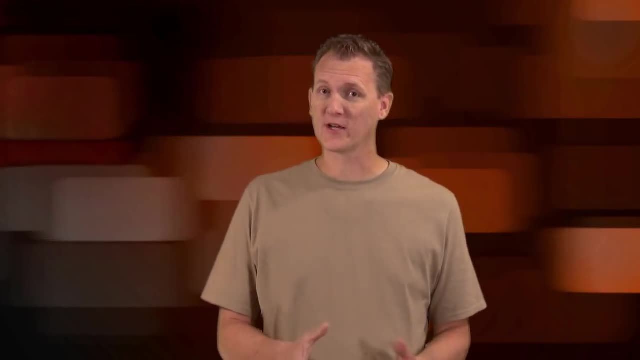 So there you have it. Multiplying fractions is easy because fractions are just another way of writing division problems. But remember, there's another way to think about fractions. We can also use fractions to represent parts of things like half a pizza, for instance. 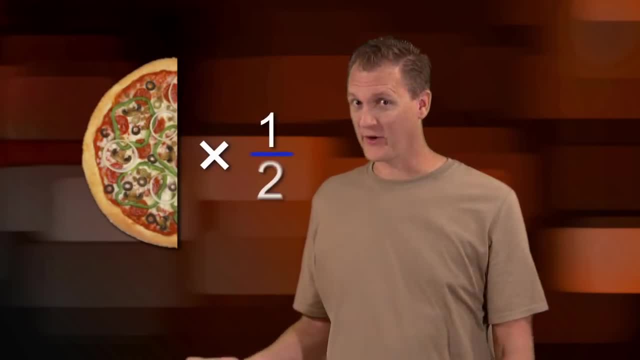 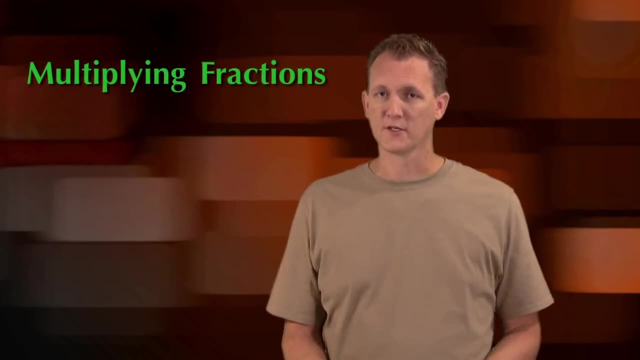 But does it make sense to multiply half a pizza by another half? Actually it does. If you're thinking of fractions as parts of something, then multiplying fractions is really like taking part of another part. For example, here's half a pizza. Now you can see that. 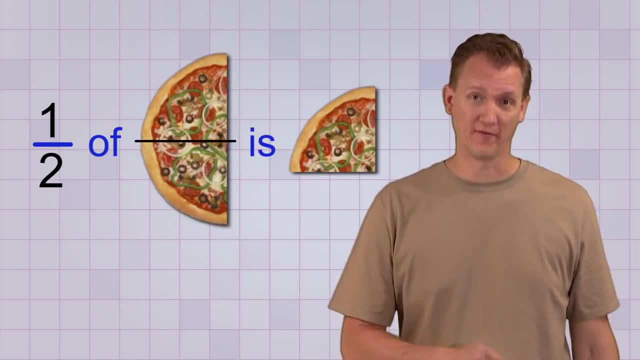 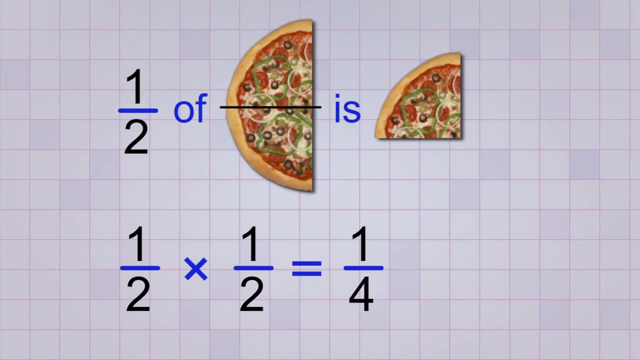 if I take one half of that half, then I get one fourth of a pizza, And if we do the multiplication, you see that we do get one fourth. So that's why you can think of multiplying fractions as taking part of another part. 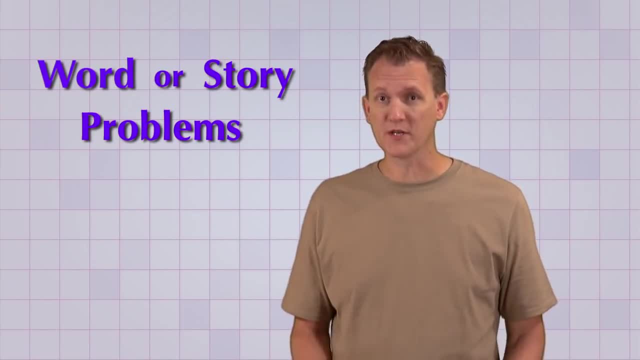 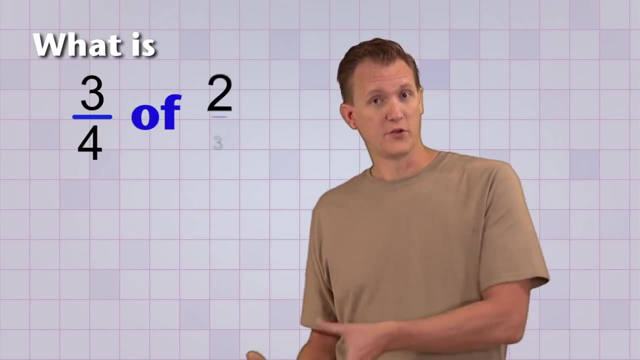 In fact, sometimes, especially in word or story problems, you'll see multiplying fractions written using the word of instead of times. They may ask: what's three fourths of two thirds? And now you know. they just mean what's three fourths times two thirds. 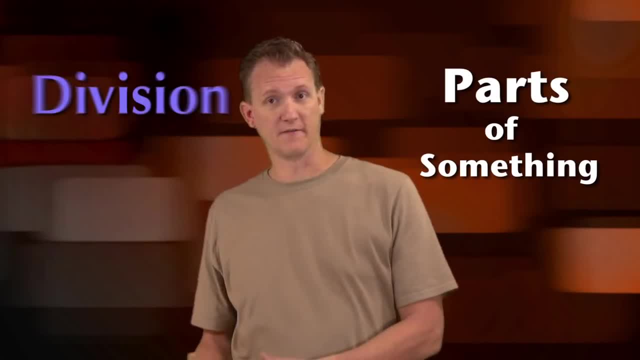 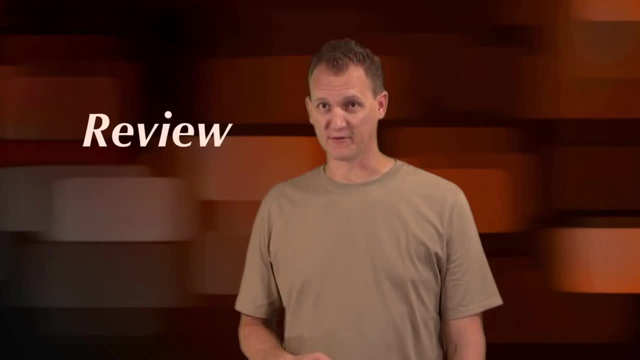 So whether you think of fractions as parts of something or as division problems, the procedure for doing the multiplication is exactly the same. Let's do a quick review of what we've learned. Multiplying fractions is even easier than adding fractions. It's easy because order. 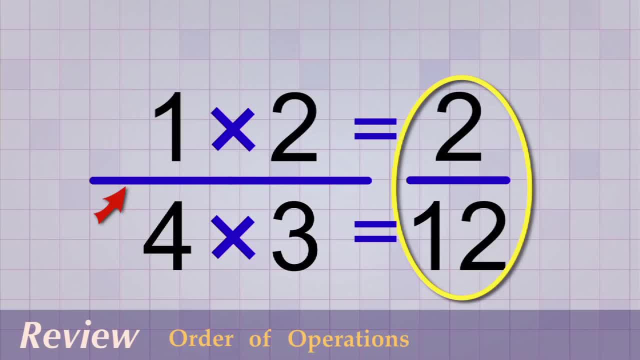 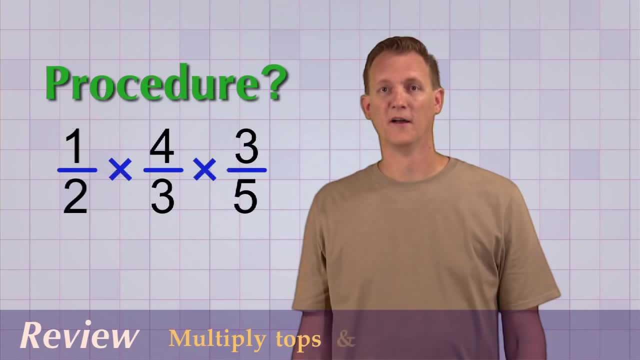 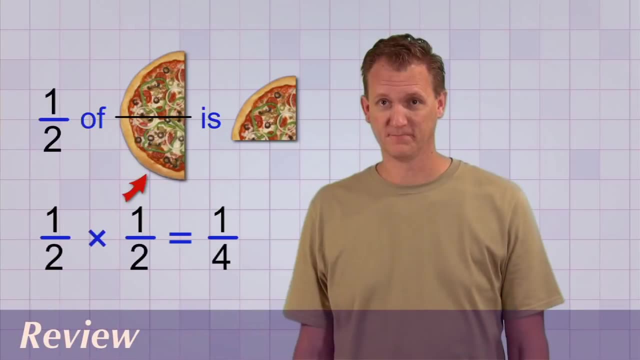 of operations says that we can do the multiplication before the division. The procedure for multiplying fractions is to multiply the top numbers to get the answer's top number and multiply the bottom numbers to get the answer's bottom number. If you think of fractions as parts of something, then multiplying a fraction by another fraction. 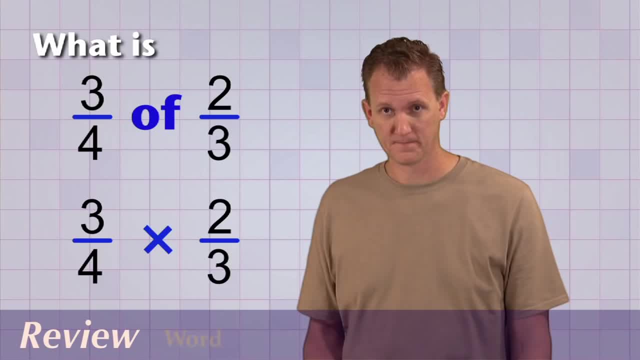 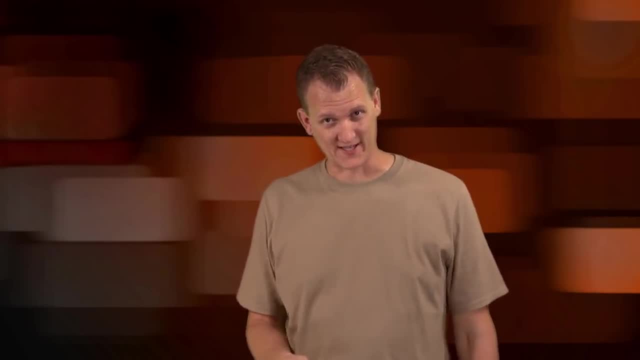 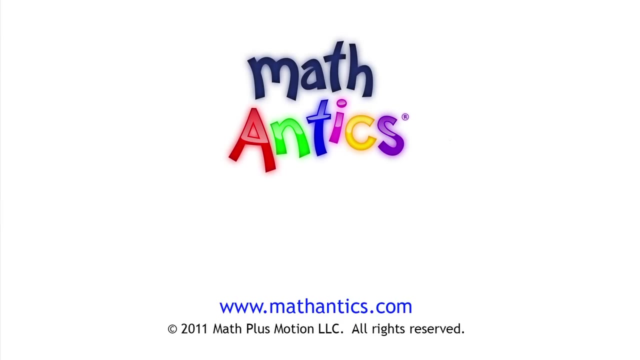 is part of a part, And sometimes, especially in word problems, you might see the word of instead of the word times. Even though multiplying fractions is so easy, it's a good idea to practice. So be sure to do the exercises And I'll see you next time.